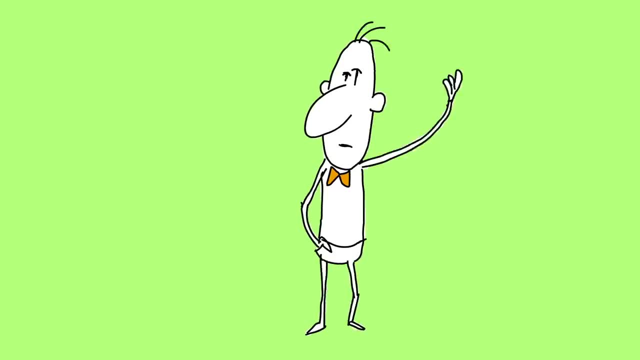 One challenge certainly lies with the complex concept of the persistence of identity: Which you is, who, The person you are today, Five years ago, Who you'll be in 50 years And when is am This week, Today, This hour? 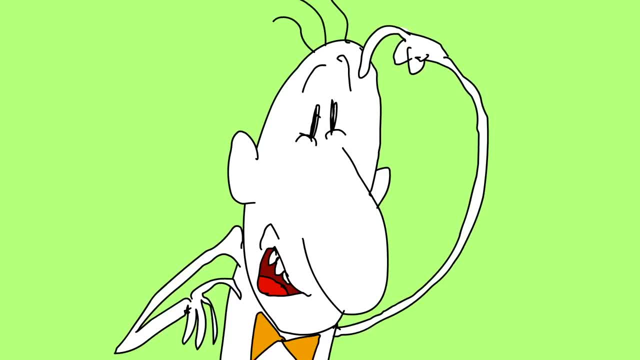 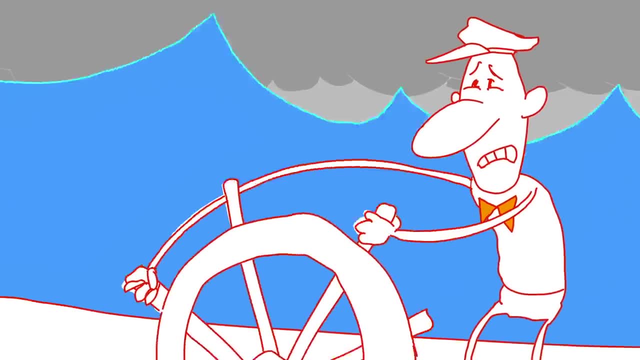 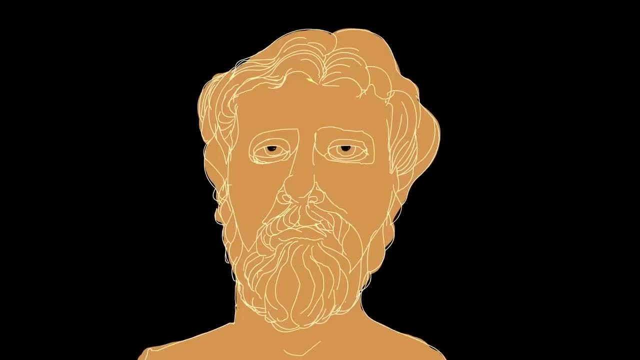 This second, And which aspect of you is I? Are you your physical body, Your thoughts and feelings, Your actions? These murky waters of abstract logic are tricky to navigate, and so it's probably fitting that, to demonstrate the complexity, the Greek historian Plutarch used the story of a ship. 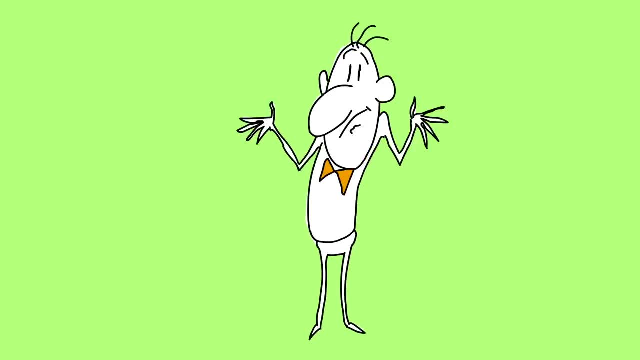 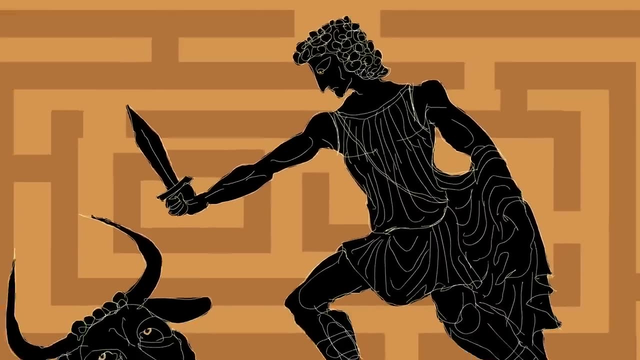 How are you I? How are you I? How are you I? As the tale goes, Theseus, the mythical founder king of Athens, single-handedly slayed the evil Minotaur at Crete, then returned home on a ship. 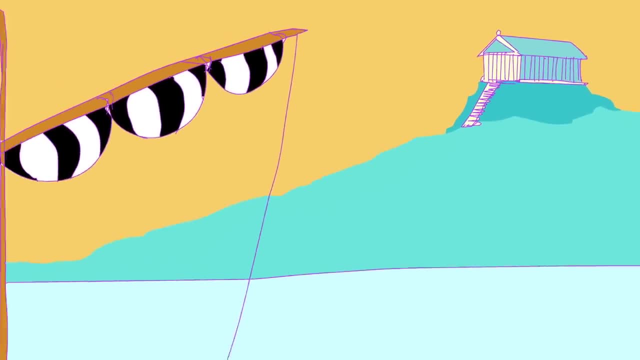 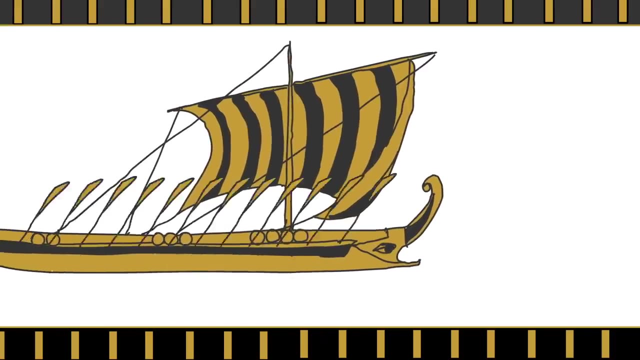 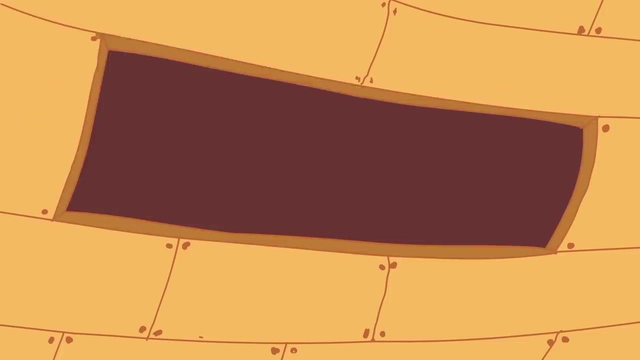 To honor this heroic feat. for 1,000 years, Athenians painstakingly maintained his ship in the harbor and annually reenacted his voyage. Whenever a part of the ship was worn out or damaged, it was replaced with an identical piece of the same material. 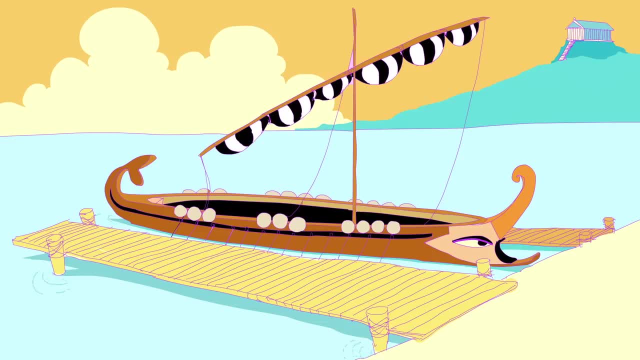 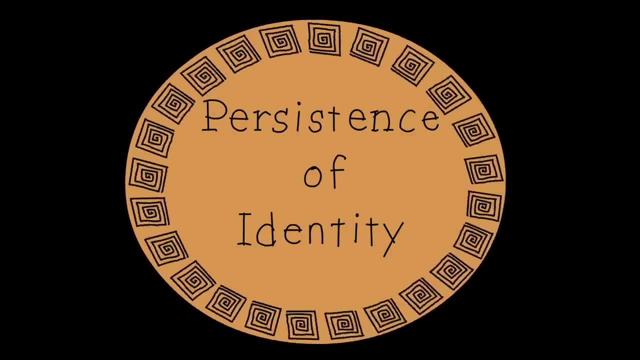 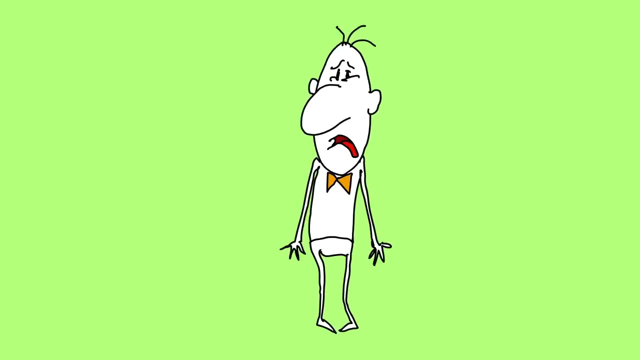 until at some point, no original parts remained. Plutarch noted the ship of Theseus was an example of the philosophical paradox revolving around the persistence of identity. How can every single part of something be replaced? yet it still remains the same thing. Let's imagine there are two ships. 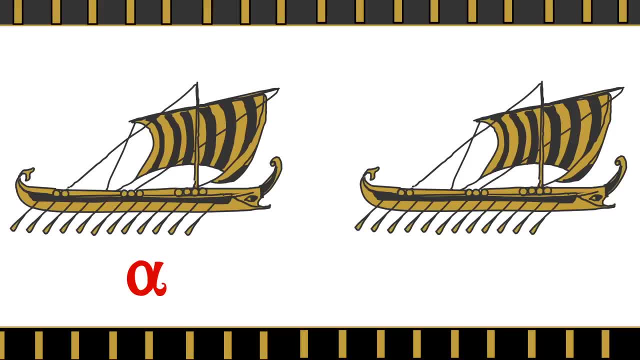 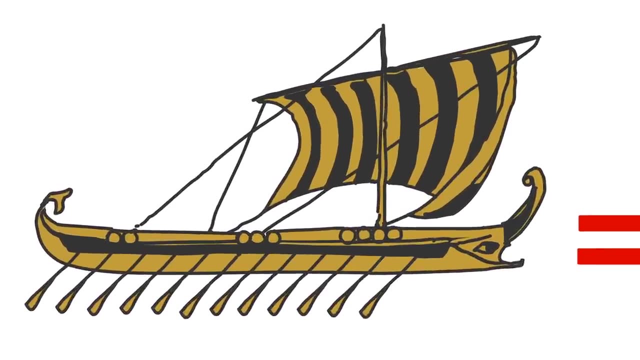 The ship that Theseus docked in Athens- Ship A- and the ship sailed by the Athenians 1,000 years later- Ship B. Very simply, our question is this: Does A equal B? Some would say that for 1,000 years there has been only one ship of Theseus. 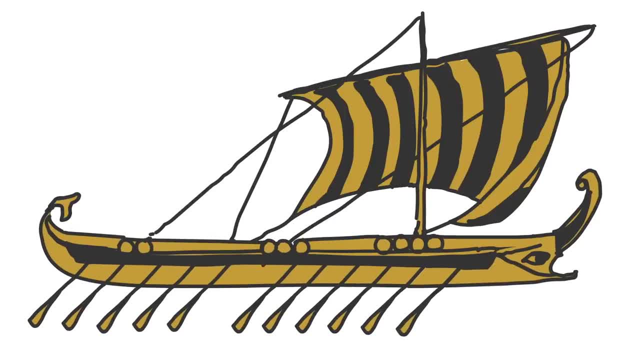 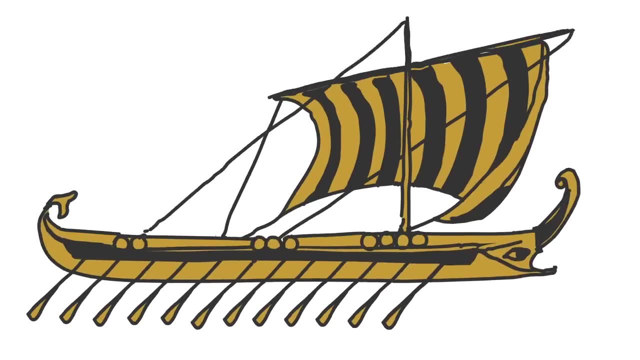 and because the changes made to it happened gradually, it never, at any point in time, stopped being the legendary ship. Though they have absolutely no parts in common, the two ships are numerous. They are numerically identical, meaning one and the same. 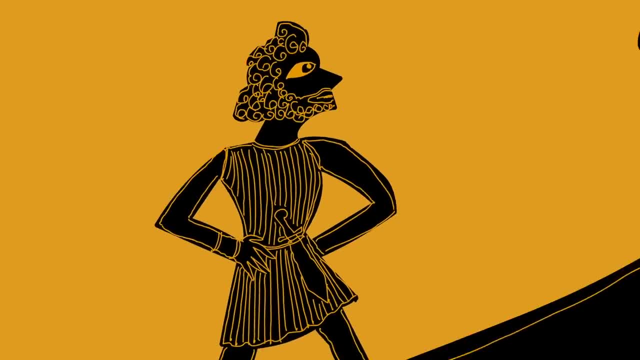 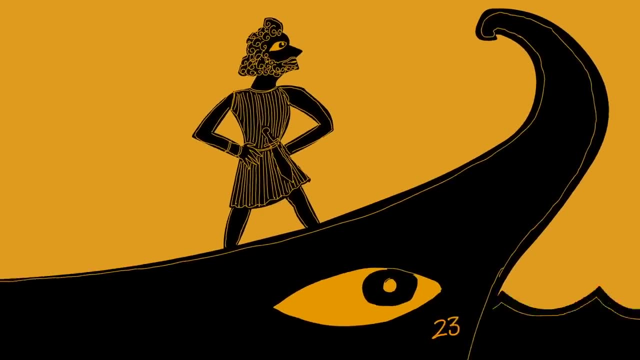 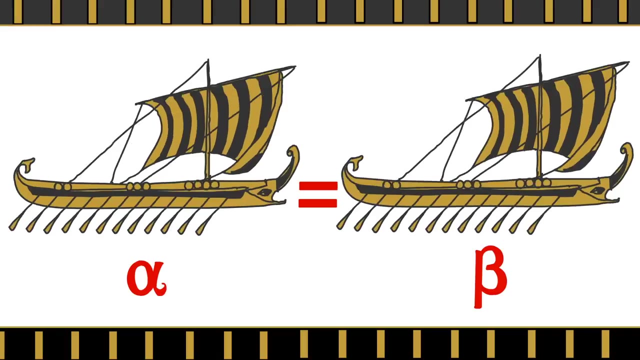 So A equals B. However, others could argue that Theseus never set foot on Ship B, and his presence on the ship is an essential qualitative property of the ship of Theseus. It cannot survive without him. So though, the two ships are numerically identical. 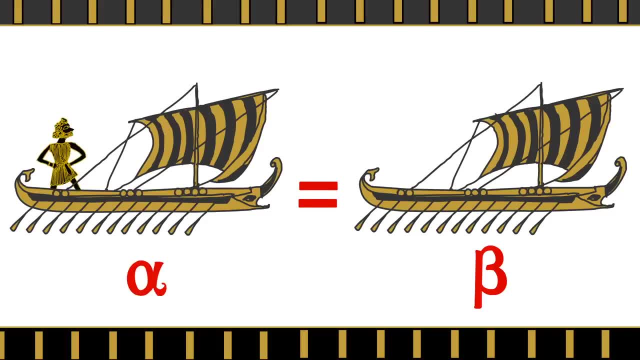 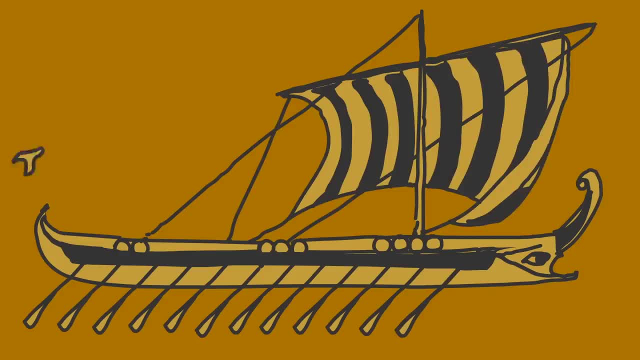 they are not qualitatively identical. Thus A does not equal B. We consider this twist. What if, as each piece of the original ship was cast off, somebody collected them all and rebuilt the entire original ship When it was finished? 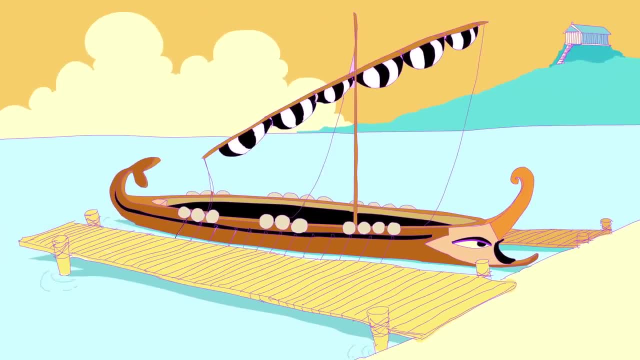 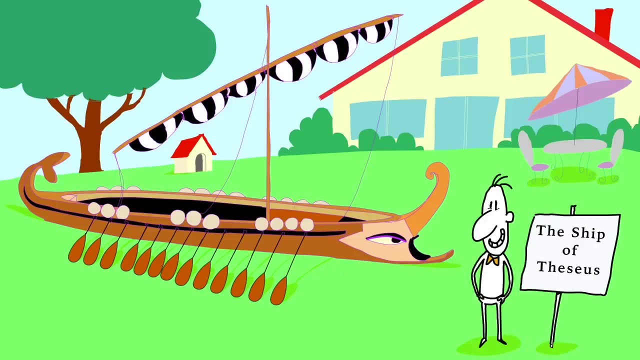 undeniably, two physical ships would exist: the one that's docked in Athens and the one in some guy's backyard. Each could lay claim to the title- the Ship of Theseus, but only one could actually be the real thing. 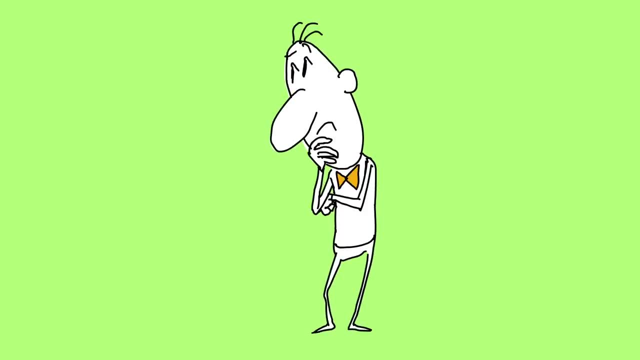 So which one is it And, more importantly, what does this have to do with you? Like the Ship of Theseus, you are a collection of constantly changing parts: Your physical body, mind, emotions, circumstances and even your quirks. 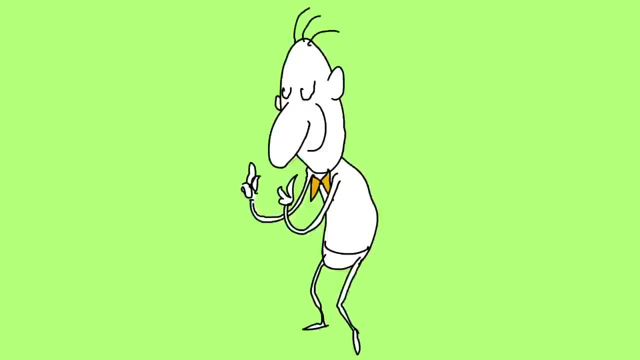 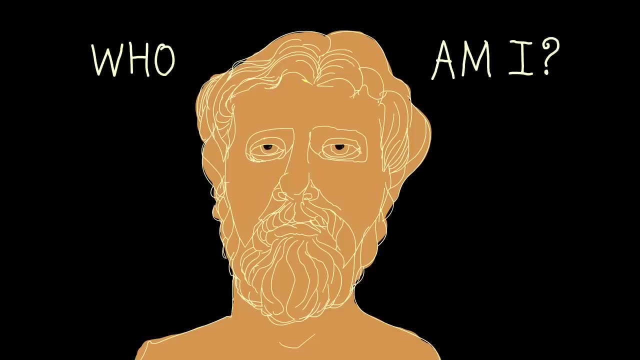 always changing, but still, in an amazing and sometimes illogical way, you stay the same too. This is one of the reasons that the question Who am I is so complex And in order to answer it, like so many great minds before you, 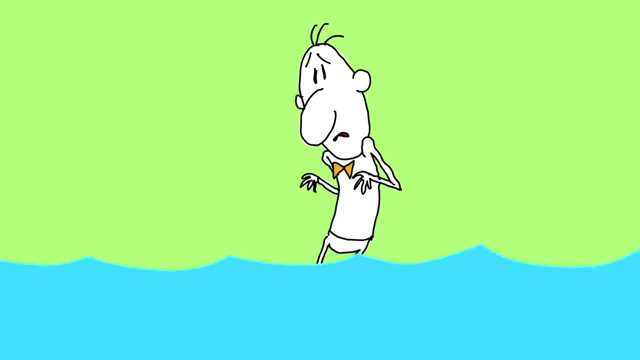 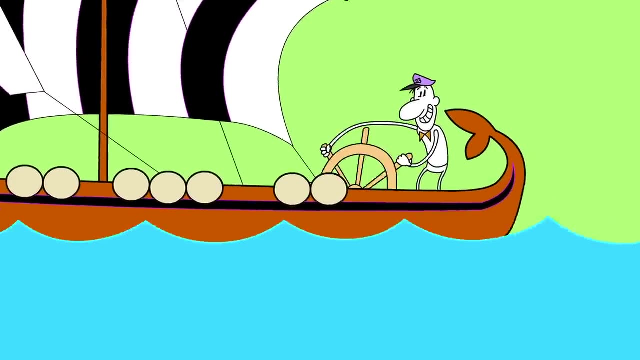 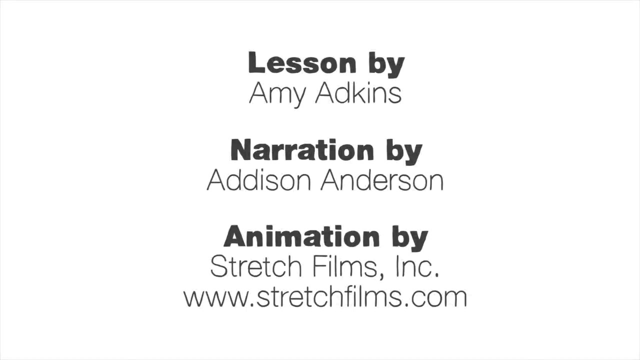 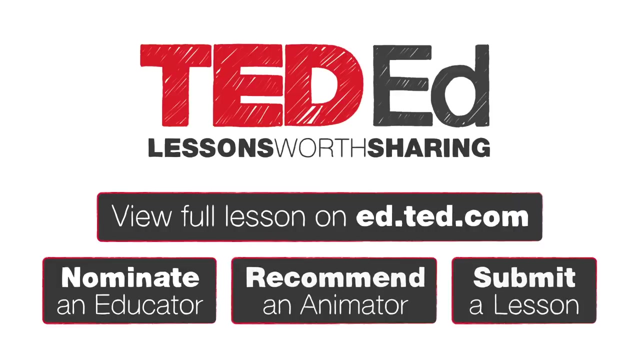 you must be willing to dive in to the bottomless ocean of philosophical paradise. Or maybe you could just answer: I am a legendary hero sailing a powerful ship on an epic journey. That could work too. I mean, you're starting all over again. You can't be too sure, especially if you're at the same page as me. Not only that, but you're also. Hopefully you'll have a good idea of what you're looking for in this. Ask a Poem or two. So it's a tough question. but I'll give it a go And, uh, I'll be more than happy to answer any one of your questions. So, thank you, Thank you All right, Thanks, Fr. So so now the next comment from our. the audience is a really wonderful question. 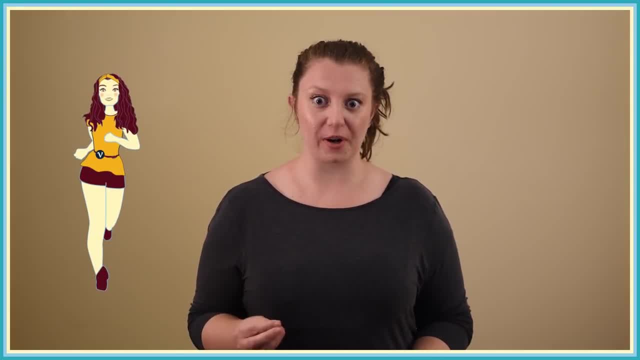 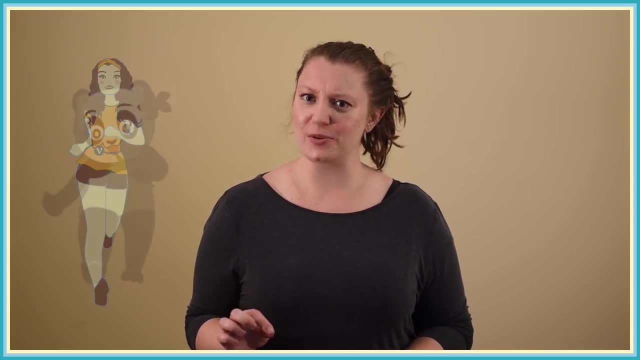 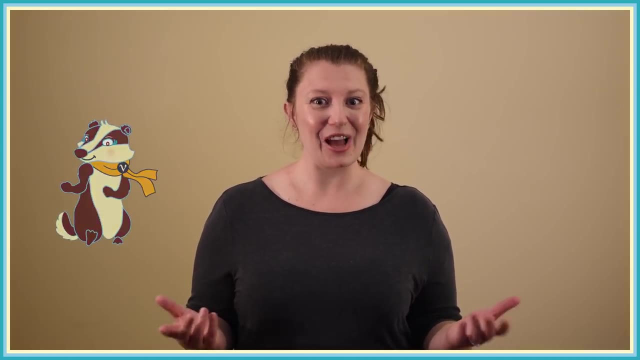 Imagine you're running a marathon. You high-five someone at the first mile marker and they see you as a human Normal. You high-five someone else at the 10 mile mark and now they see you as a panda. And when you high-five someone at the finish line, you're a honey badger. Bizarre, Yes, But this is.